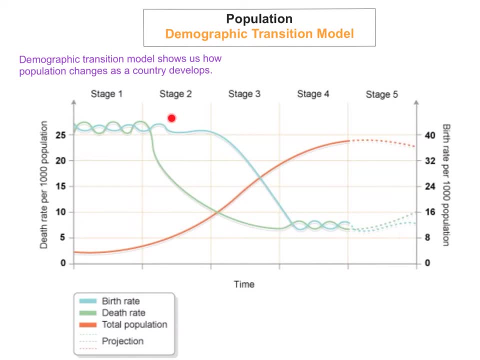 that birth and debt rates are very high. In stage two, the debt rates will start to slow down a bit. okay, So the debt rates, the green line, starts to slow down a bit, But birth rates will still remain very, very high. So what does this mean? Well, if the same. 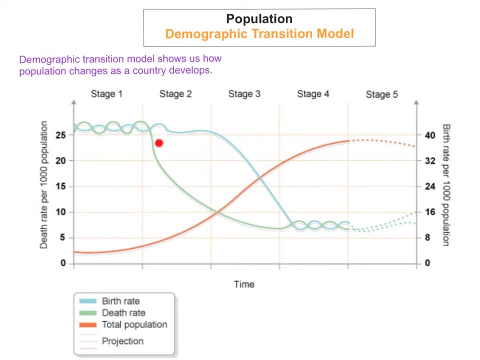 if there's a very high birth rate and the debt rates have slowed down a lot, what's going to happen here is the population starts to going to increase. There's a lot more people being born than are dying. therefore, the population will increase. In stage three, the birth rate starts. 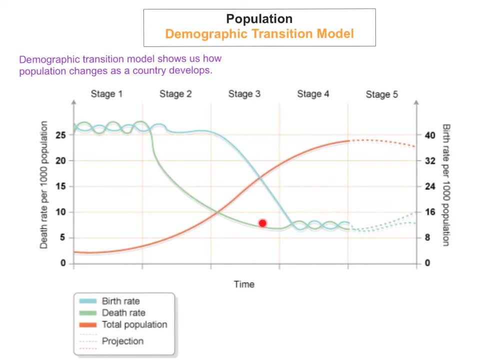 to decrease and the debt rate continues to decrease as well. Why is this? Well, the improvement in technology, improvement in health care and sanitation, better medical care and education as well, and better use of family planning and contraceptive methods gives people better understanding and therefore they have less children and they also let people die. 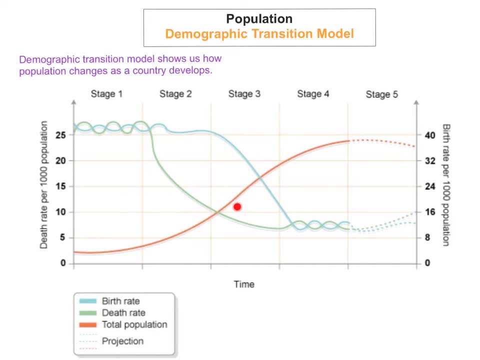 So what happens now is the population still increases, but it's starting to slow down. When you get to stage four, the population, the population cycle changes okay. So the birth rate will continue to decrease and in stage four, the debt rate- actually the birth rate and debt rate- 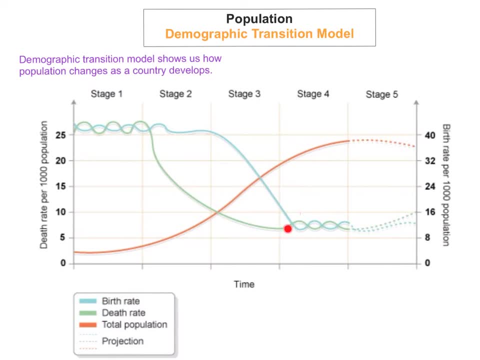 will fluctuate. So at certain stages, in times of stage four, you'll have an increase in population and also a decrease in population, And when you get to stage five, this is when the death rate actually exceeds the birth rate and stays that way. So what happens here in stage five is: 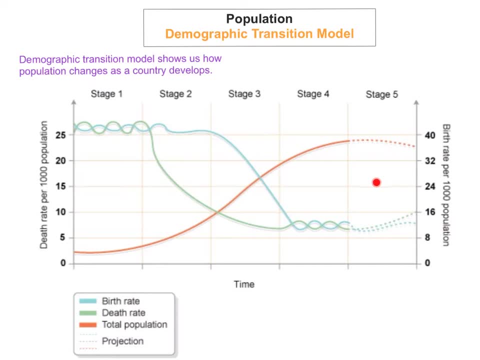 population starts to decrease. Now it's not very fast, it's a slow decrease. So you can see this line here. it shows when population has increased dramatically And then, when we get to about stage five, it starts to slowly decrease. Okay, so I'm quickly going to look at each of the stages and 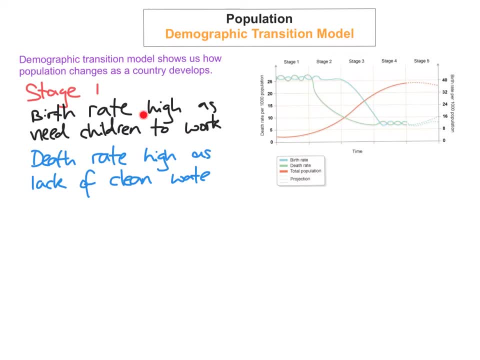 just as I wrote down here just one point for each one. So stage one is the fluctuation stage. both birth rates and debt rates are really high. Birth rates are high because they need children to work. they need to send them out. Also, they need children to look. 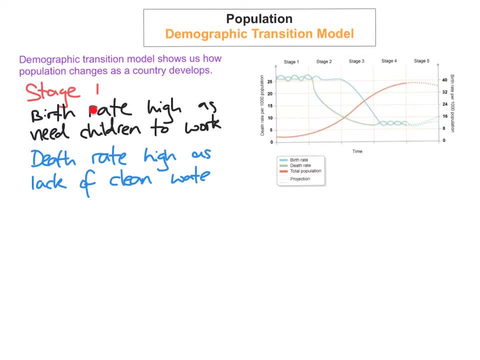 after their parents when they get older, And also not many children actually survive. So they have quite a lot of children in stage one. The debt rate is really high. there's a lack of clean water, there's a lack of sanitation, they lack education, they lack family planning and lack basic medical. 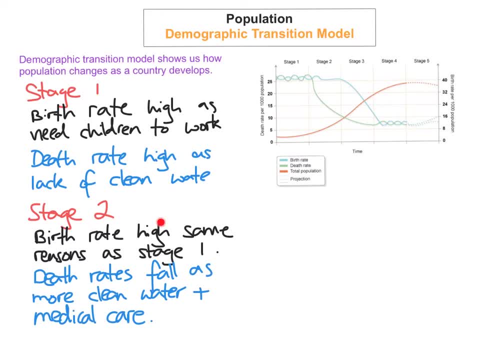 care. So in stage two, birth rate remains high because of the same reasons as we had in stage one. they need children to work, they need children to look after their parents when they get old. Debt rate falls dramatically, though. debt rate falls dramatically Why? Because there's more. 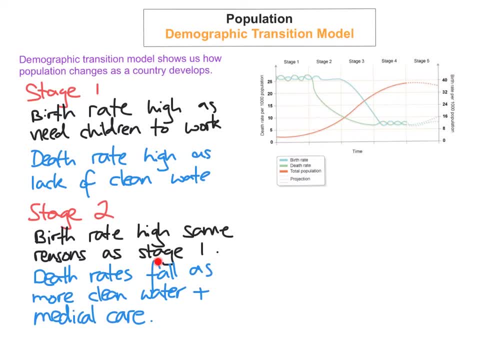 access to clean water, medical care is improved and there's a better sanitation. In stage three, the birth rate falls dramatically. This is because the improvement of technology, such as helping out in the farms, machines and tractors, can do the work, So they don't need to have as many. 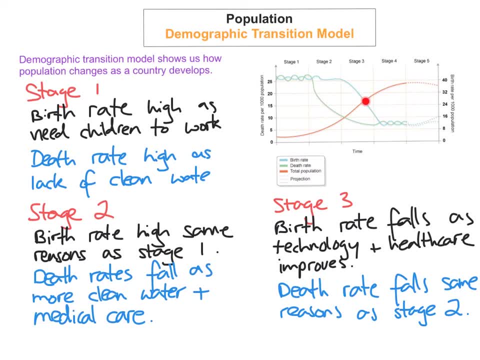 children, Family planning and technology. no, family planning and education become is improved, So people know more about family planning and contraceptive methods. Healthcare also improves, so infant mortality is reduced And in stage three the debt rate does, continues to. 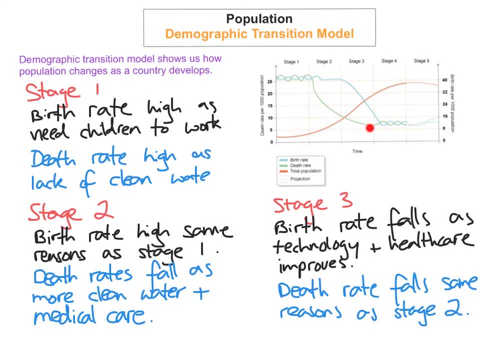 decline, but not as rapidly as it did in stage two. It starts to ease off, but it still is declining, and for the same reasons as in stage two: because there's more access to cleaner water, medical care is improved, improvements in sanitation, better education of foods and what they should be doing. 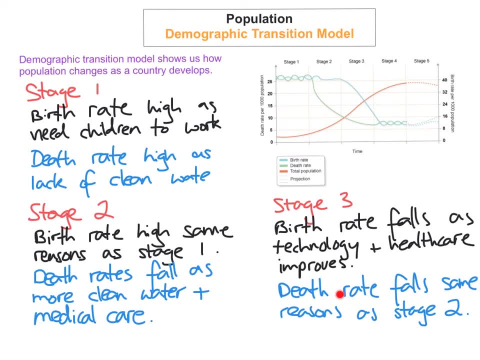 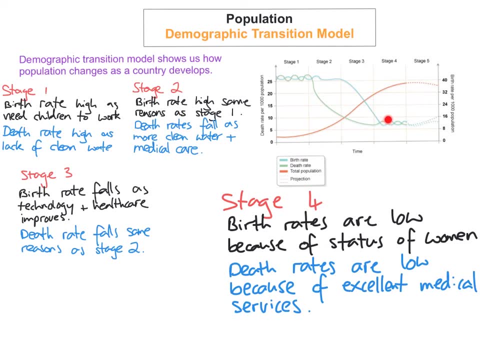 And what people should be eating And what healthy diets and so on. In stage four, birth rates are low because the role of women have changed, the status of women has changed. Women are now working from outside the home. they're not using, they're not focusing on that traditional role of 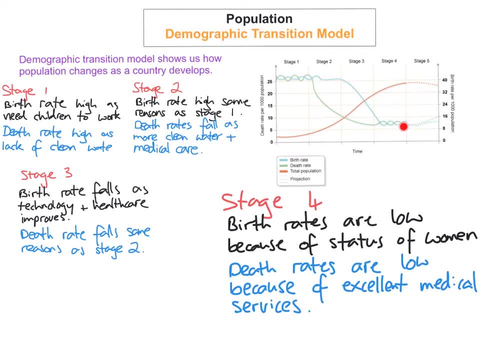 just looking after children And there's more family planning and they're better educated. And some- some women- are just leaving having children till later on in the life- Like life, so they don't have as many children. The debt rates are also low because of excellent. 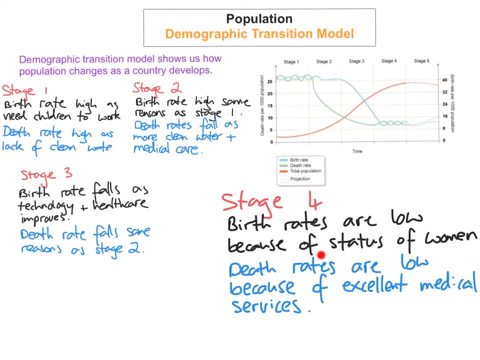 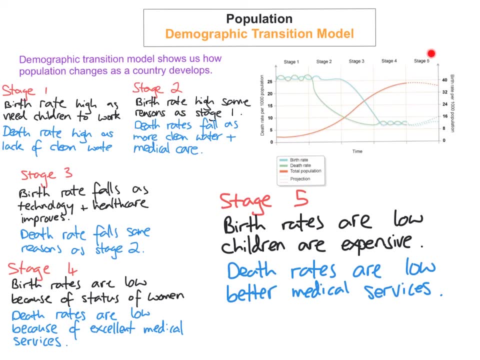 medical service, improved technology and overall better sanitation and access to clean water. And the very last stage, stage five, you can see that the population is starting to decrease and this is because birth rates are very low and it's because one of the reasons is because 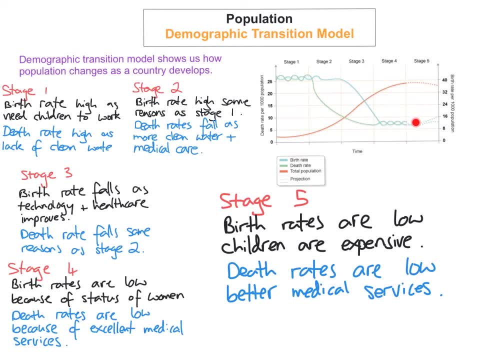 children are seen as expensive. family planning is really practiced in stage five of a country, and you also have the fact that women have huge, really good status within society. The role of women is completely different in stage five compared to stage three or two, and they 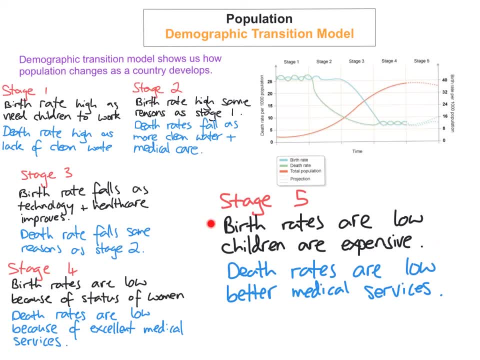 are now better educated, they secure higher roles in society and jobs, and they just don't have as much time to have as many children. Debt rates are low, and this is because the population is starting to decrease, and this is because of better healthcare, medical services. 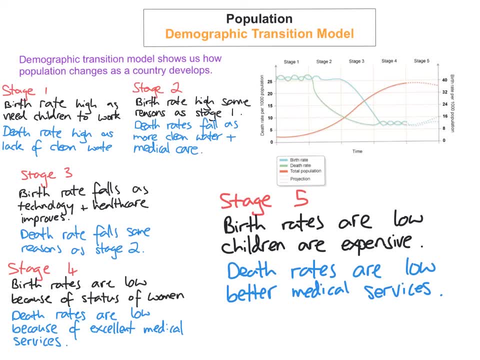 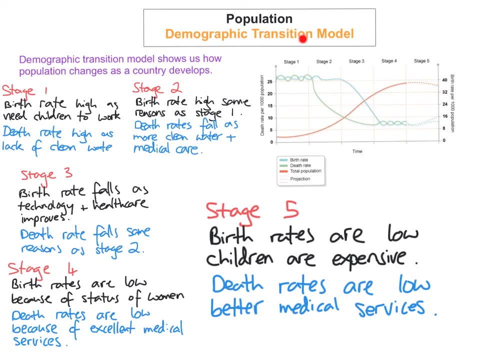 such as nursing homes, and also people are living longer. If you'd like to know an example for each one of these stages, stage one would be like a tribal group in Africa. stage two would be the country of Mali. stage three would be the country of Brazil. stage four would be us, the Republic of Ireland, and stage 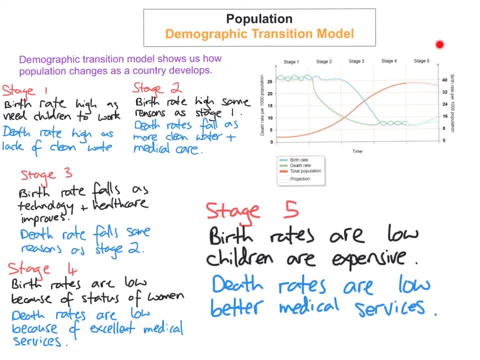 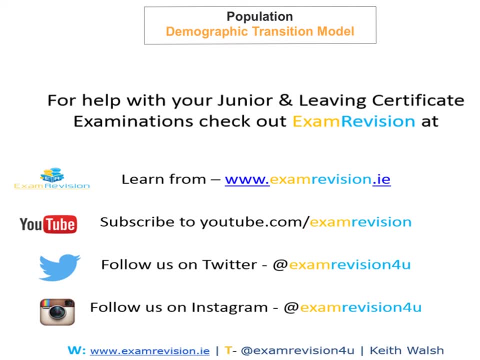 five would be the country Germany. Okay, so that's it for today's tutorial on the demographic transition model. It's really, really important that students understand the demographic transition model. You need to understand what happens at each of the five stages and you need to understand why. 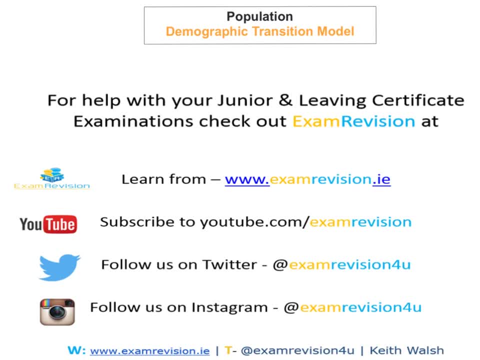 these things happen. at each of the stages You need to know what causes it, what's improved, what's made the birth rate decrease, what's made the birth rate increase and so on. So the debt rate increase and the debt rate decrease, and what is the overall result and the impact. 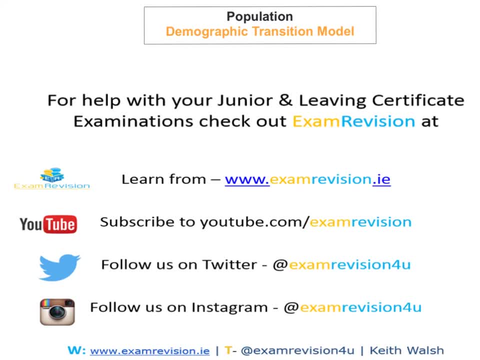 it will have on the economy. If you enjoyed my video, if it helped you, can you please, please, can you subscribe to my YouTube channel, youtubecom forward slash exam revision? You can check out more videos on the YouTube channel and also on my website and, if you would like to just keep up to date, 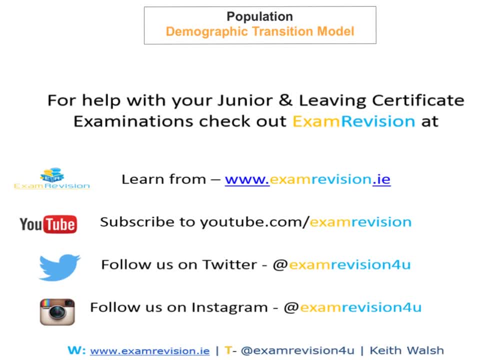 with all the latest news. you can follow us on Twitter and Instagram at exam revision for you, Thank you.